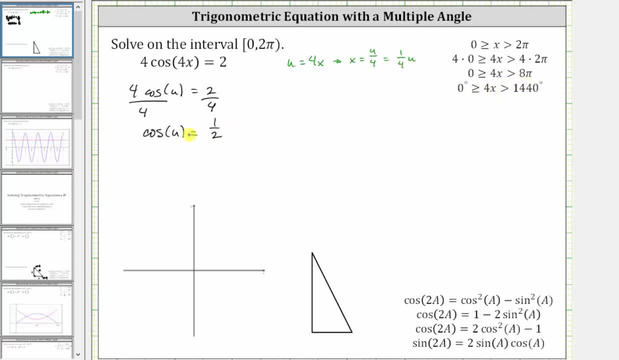 So now we need to find all the angles from zero to eight pi that have a cosine function value of 1 1⁄2.. Having a cosine function value of 1 1⁄2 should remind us of a 30-60-90 reference triangle. 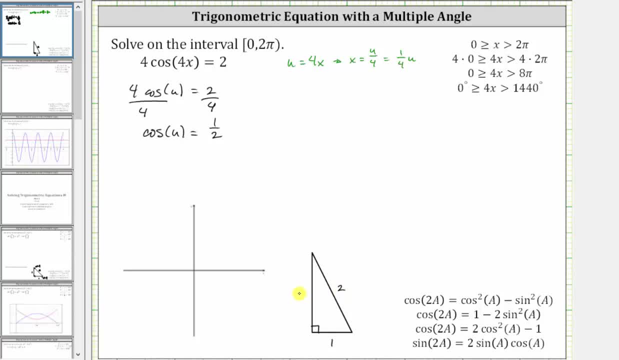 where we label the short leg one, the hypotenuse two and the longer leg square root three, where the small angle is 30 degrees, or pi over six radians, And the other acute angle is 60 degrees, which is equal to pi over three radians. 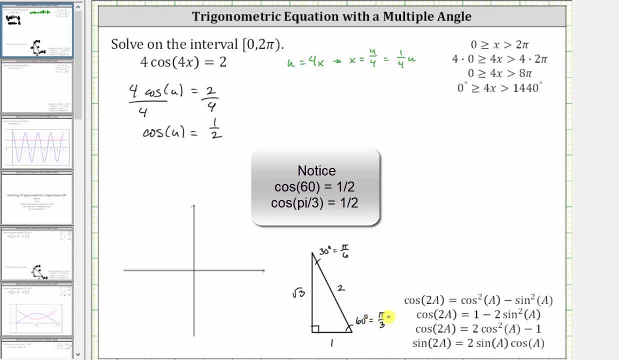 And the other acute angle is 60 degrees, which is equal to pi over three radians, And the other acute angle is 60 degrees, which is equal to pi over three radians. Next, on the coordinate plane cosine theta is equal to x divided by r, and since x is 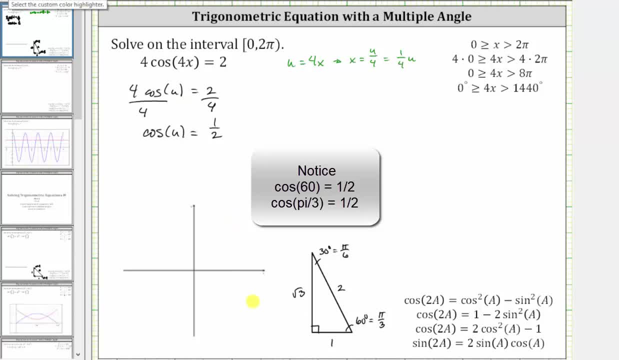 positive in the first and fourth quadrants. we will now sketch a reference angle of 60 degrees in the first and fourth quadrants and also sketch the reference triangle. Here's the reference angle of 60 degrees in the first quadrant. Here's the reference triangle where this angle here is 60 degrees. if we want pi over. 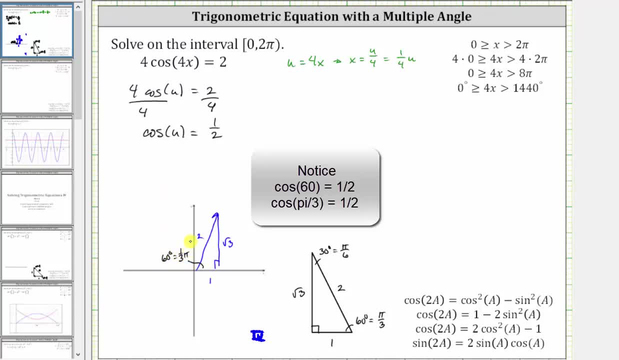 three or one-third pi radians. and now let's sketch the reference angle of 60 degrees in the fourth quadrant, which is here, and here's the reference triangle. So in standard position this angle is 300 degrees if we want five-thirds pi radians. but again, we're looking for all. 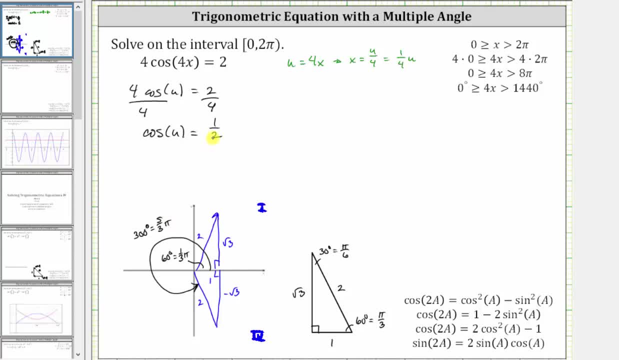 the angles that have a cosine function value of one-half, from zero to eight pi. so we will let u equal one-third pi radians plus multiples of two pi, which will give us coterminal angles to one-third pi radians. So that's what we're looking for. 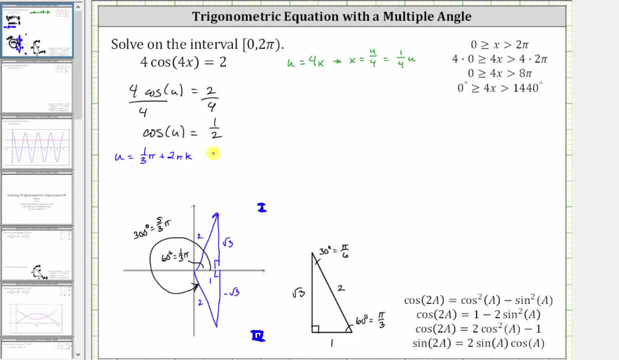 So we'll say plus two pi times k, where k is some integer. This would be all the angles that are coterminal to one-third pi radians, and we can also have u equals five-thirds pi radians plus two pi k. Let's go ahead and list all the angles u that have a cosine function value of one-half from. 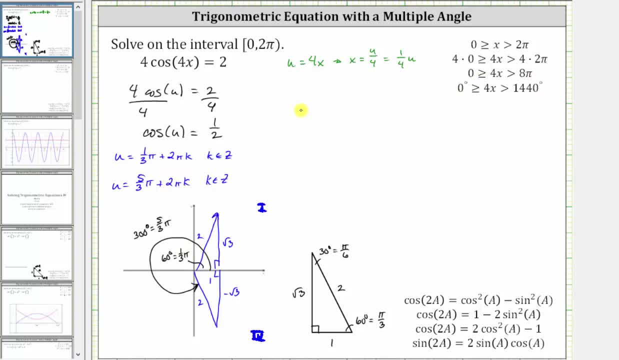 zero to eight pi. We would have u equals equals, one-third pi, as well as one-third pi plus two pi, one-third pi plus four pi and finally, one-third pi plus six pi. The next angle would be one-third pi plus eight pi, which would be greater than eight. 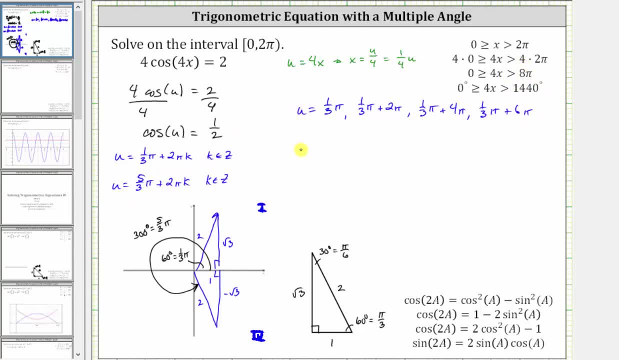 pi And then, starting at five-thirds pi radians, we have u equals five-thirds pi plus two pi, then five-thirds pi plus two pi, five-thirds pi plus four pi and five-thirds pi plus six pi. The next angle would be more than eight pi radians. 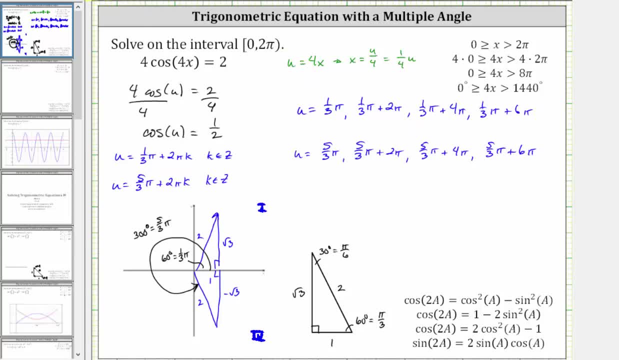 And now let's go ahead and determine these sums. where two pi or two pi over one is equal to six-thirds pi, So we're really adding more than one-third pi. Okay, So we're going to use multiples of six-thirds pi to find the coterminal angles. 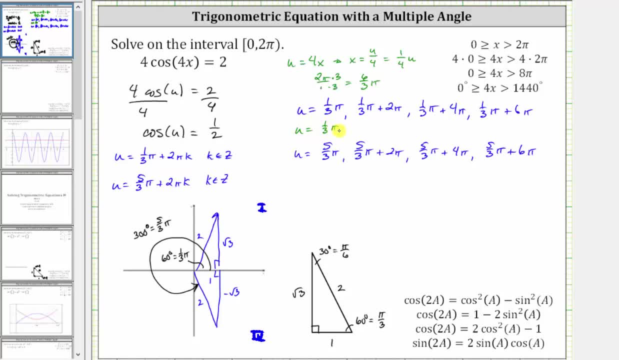 So here we have: u equals one-third pi, and then one-third pi plus six-thirds pi is seven-thirds pi. And then one-third pi plus four pi is the same as seven-thirds pi plus six-thirds pi, which is thirteen-thirds pi. And then, finally, one-third pi plus six pi is equal to thirteen-thirds pi plus six-thirds. 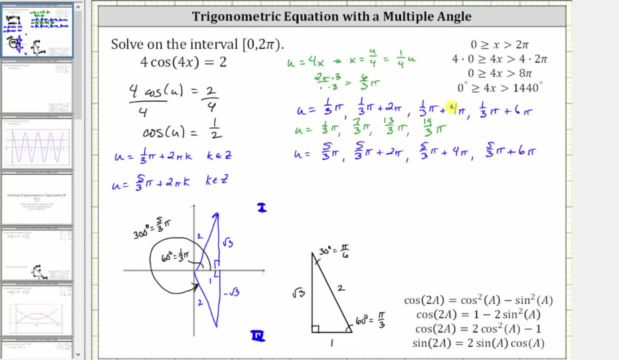 pi, which is nineteen-thirds pi. And now we'll do the same, starting at five-thirds pi, where we have u equals five-thirds pi, and then five-thirds pi plus six-thirds pi is eleven-thirds pi. and then five-thirds pi plus four pi is eleven-thirds pi plus six-thirds pi, which is seventeen-thirds pi. 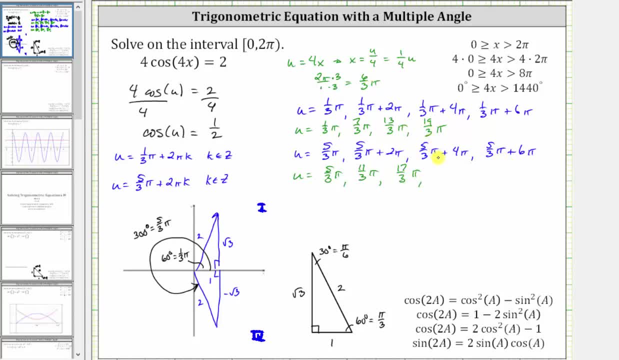 Then the last angle is seventeen-thirds pi plus six-thirds pi, which is twenty-three-thirds pi. Now we're not quite done yet. These are the eight solutions in terms of u. but remember, we're trying to solve the equation for x, not u. 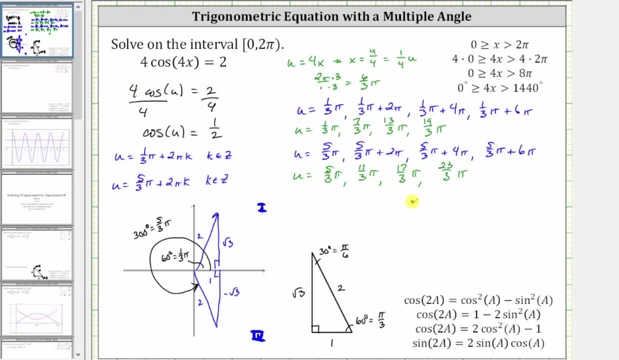 and remember, x is equal to 1 4th times u. So if x is equal to 1 4th times u, to solve the equation for x over the interval from zero to two pi, we need to take each of these eight angles.